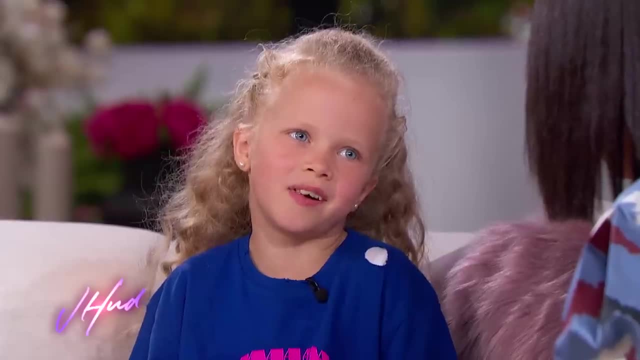 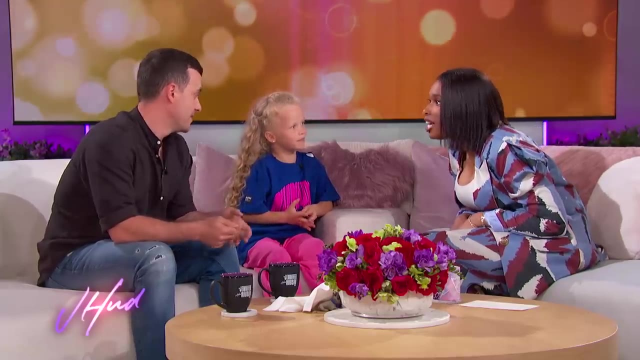 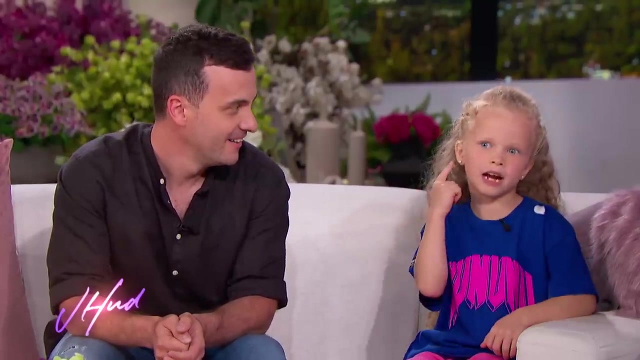 Can you tell me how long you've been dancing? When I was three years old? Yes, Yes, Actually. she began dance when she was seven months. okay, Seven months, You can tell how you begin. I sit in baby car and I hear music and I like do-do-do-do-do. 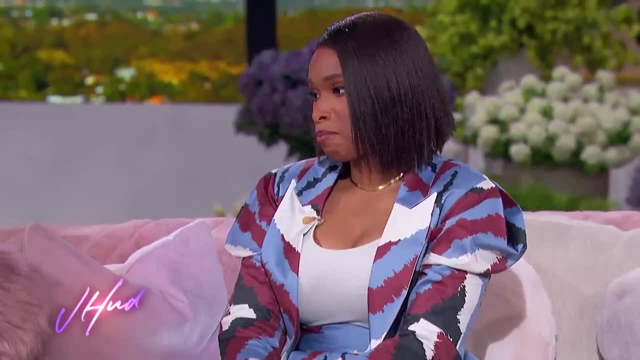 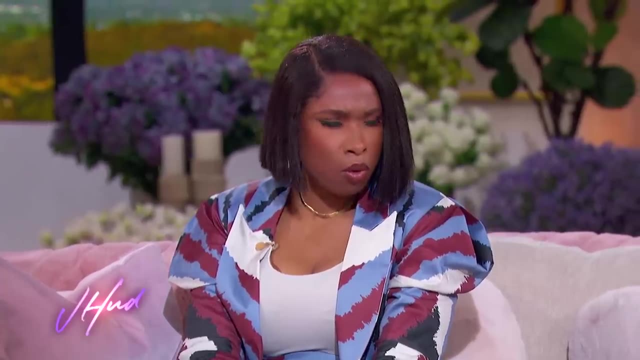 Oh my God, Tell me, what do you love most about dancing? When I dance, you feel freedom, you feel happy, you feel power. What would you say she gets the dancing from? Do you dance? You know where does she get it from? 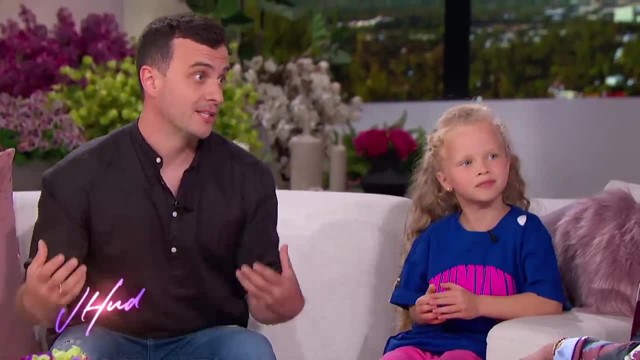 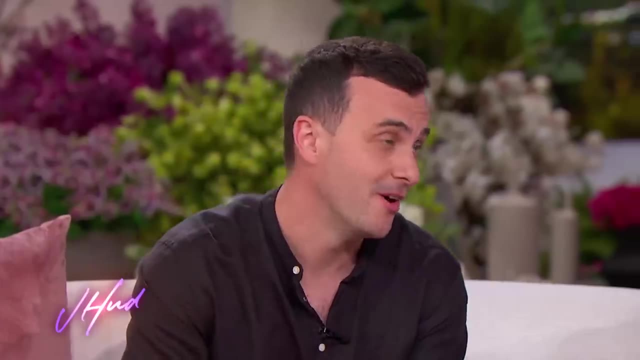 We are dance family, Me and my wife. we are dance teacher. We have a special program to teach children and we begin from Yesenia. It was Yesenia when she was very young and she danced old styles, But her feeling, it's only. 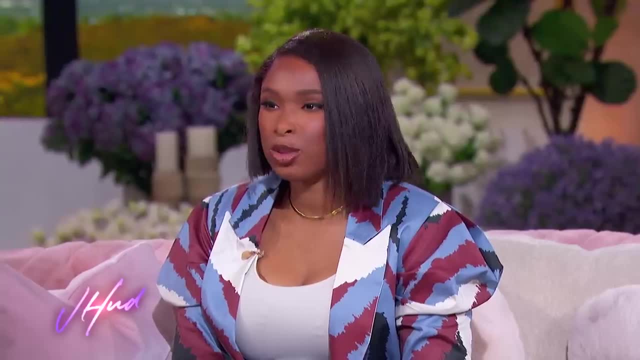 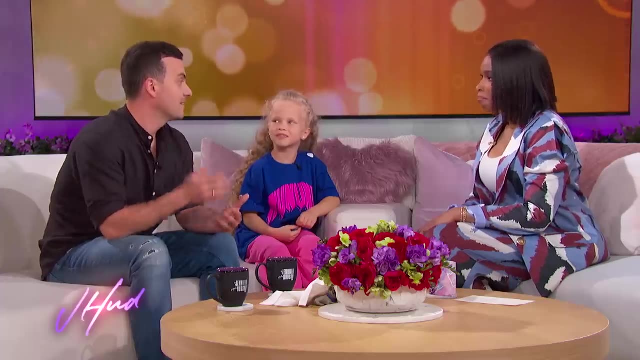 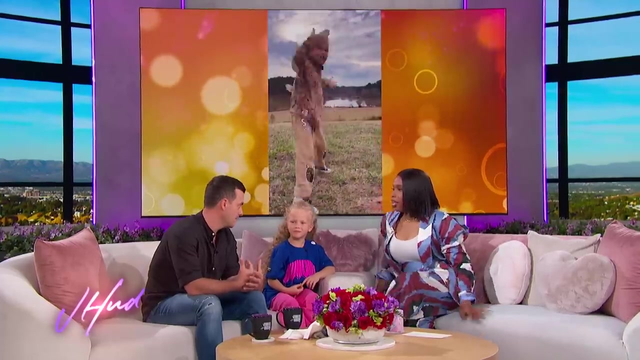 From here it's, It's so natural, it's a gift. Yes, it's like Definitely You never can teach this. It's from inside, It's from my heart, You can tell it's from your heart When she begin dance, she listen music, she feel music and from inside is go on her face. 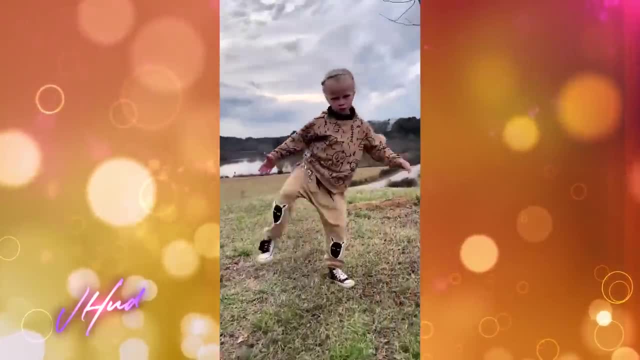 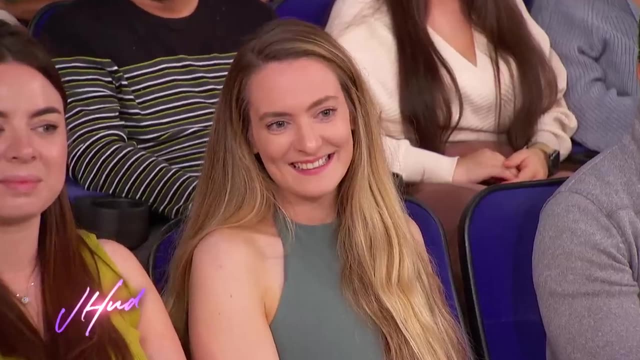 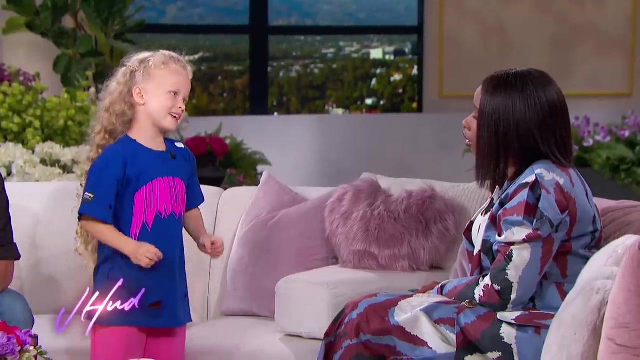 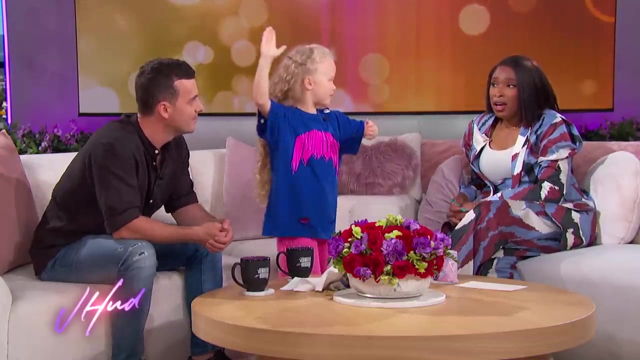 Yeah, that's why she dance like this and it's like Cool. And what is your favorite style of dancing Ballet? You have only this position and only this hands. When you dance tango, Dance tango with me. and when you hear music, tango, you dance only. 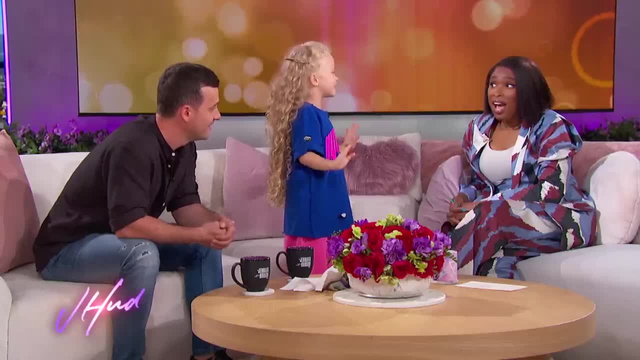 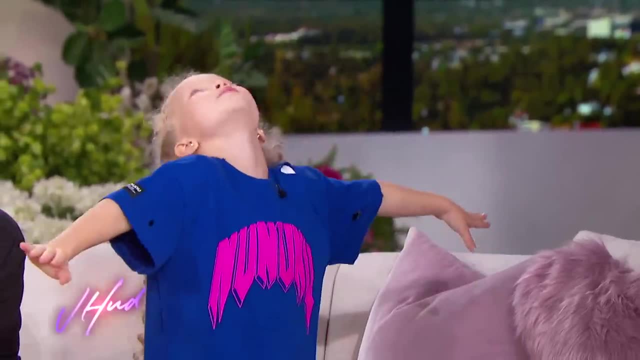 And when you dance contemporary, And when you dance contemporary, Contemporary is so slow and you go one, two, three, four. And when you dance hip hop, Yes, yes, You can dance like this. Oh, You can dance like this. 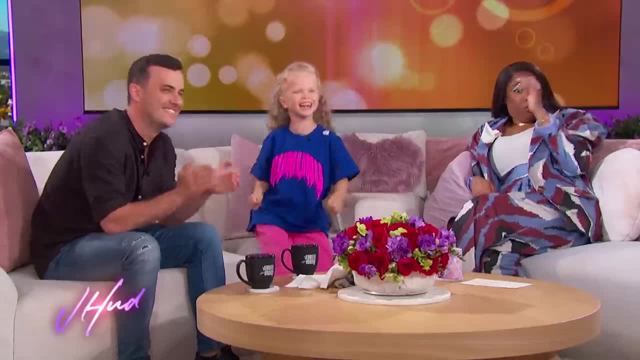 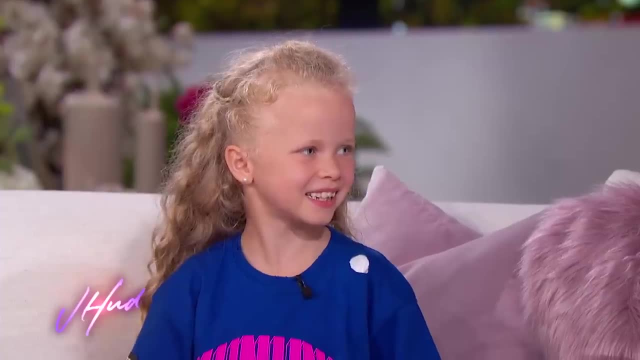 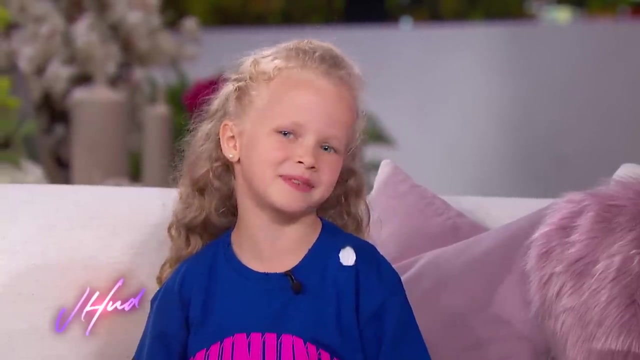 And you can dance like this. That was a. You know your stuff, Oh my God. Now I also heard you have some pets at home. Yes, I have big fat cat I'm sorry for have. That's your cat. 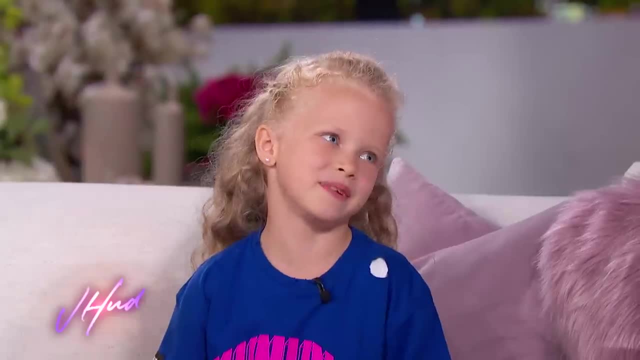 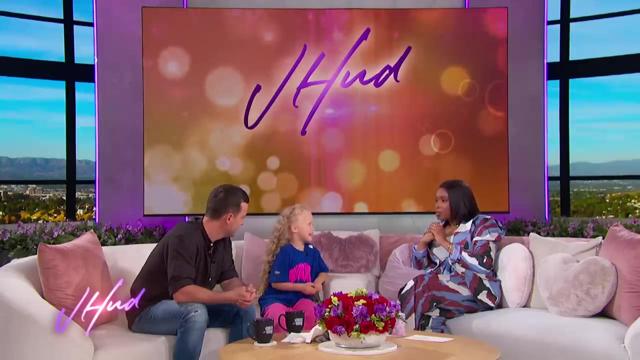 And That's your cat. Yes, What's the cat's name? Marcel Amin. Oh my God, He's so fat. I love him. I hear you have a cat. I have two cats. One of them is really fat too. 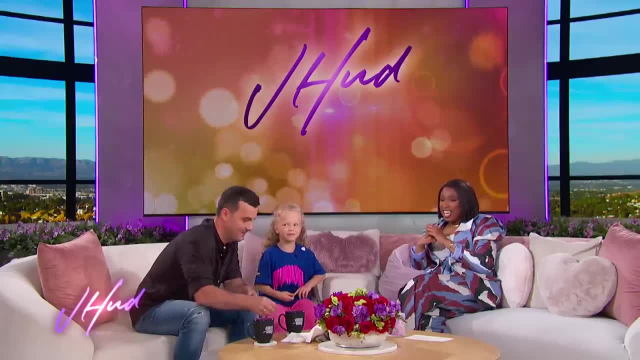 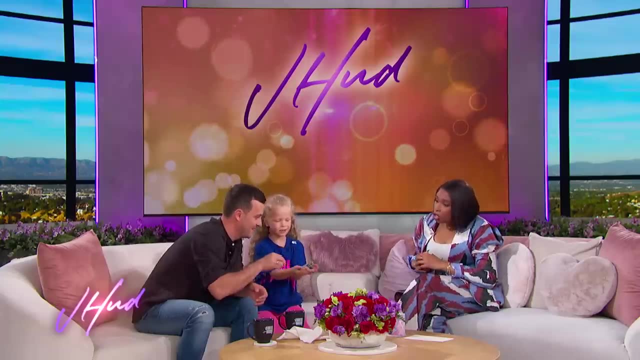 That's Chrisabella, Okay, okay, You brought me something Uh-huh, And I can make something for you. You made. You said this: Oh my God, It's, It's, It's, It's, It's. 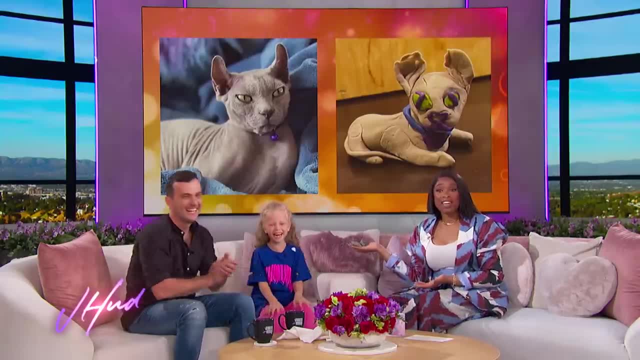 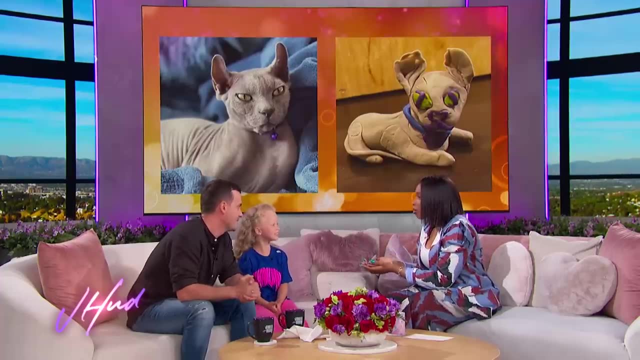 It's, It's. Oh, my God, That looks like my cat. That looks like my cat. Yes, Thank you. Oh, he's gonna love this. Y'all see that. Yeah, we Thank you so much for this. 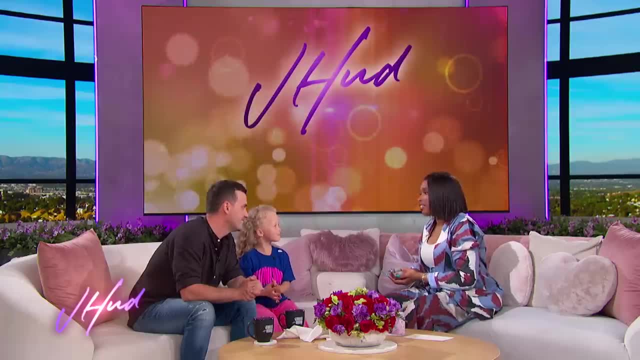 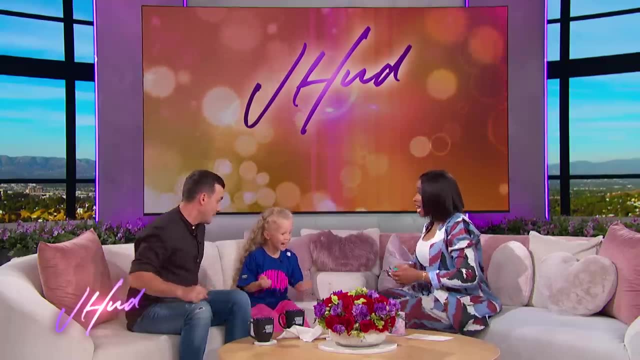 Okay, You know, You know we can't have you here and you not dance for us. Will you dance for us? We would love Dance, Dance, Oh my God. Okay, Can you go dance for us now? Okay, 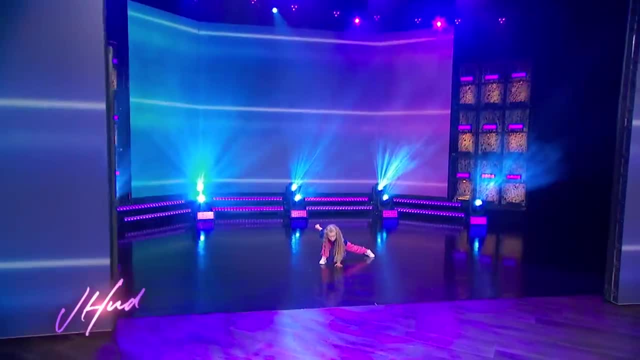 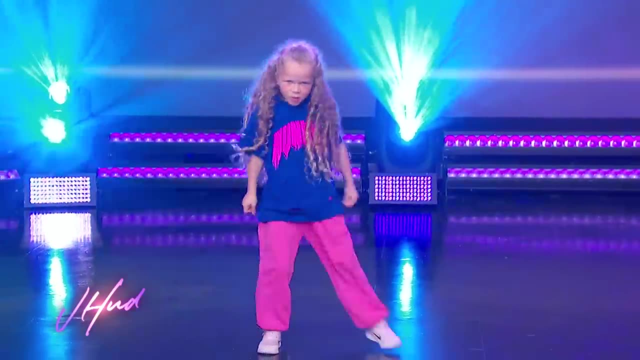 Yes, Yes, Yes, Yes, Yes, Yes, Yes, We'd love to dance for us. Stuntie, Stuntie, Stuntie, Stuntie, Stuntie, Misty you, What Misty you? 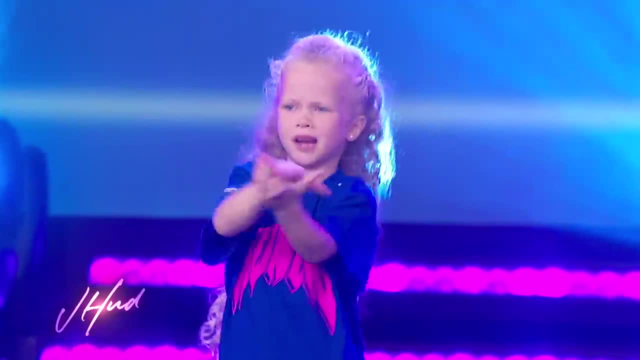 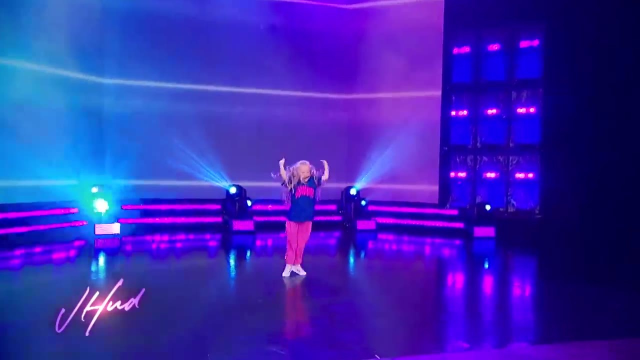 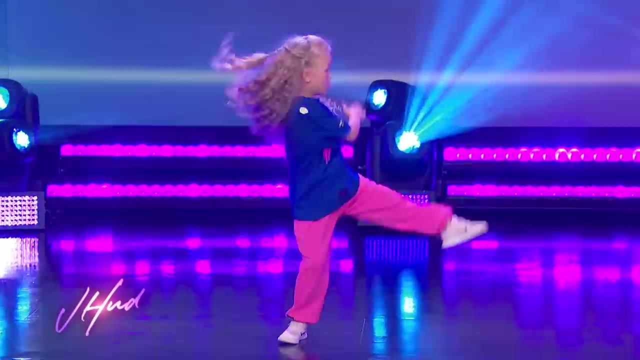 Misty, you, Where are you looking? Okay, Okay, Okay, Oh, Here we go, guys, That's the beat. Here we go. Oh, banging bells. How do you like my— Yeah, You actually like my—. You find me funny. 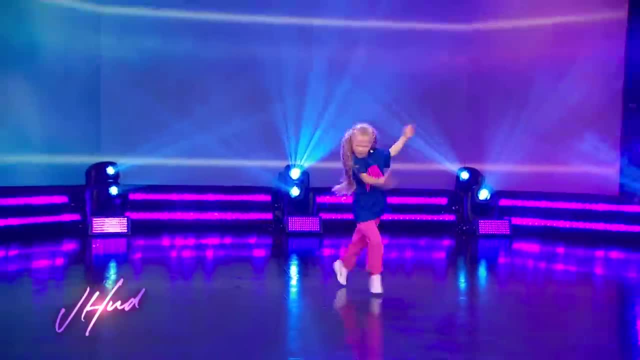 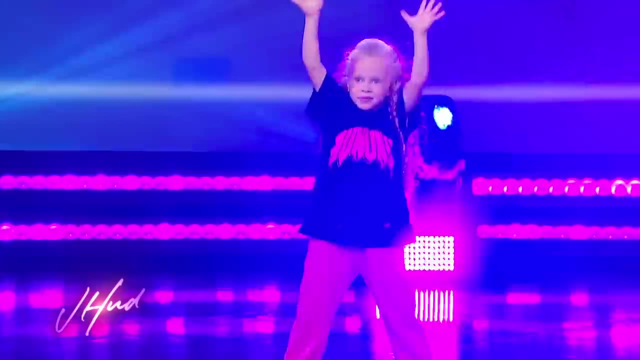 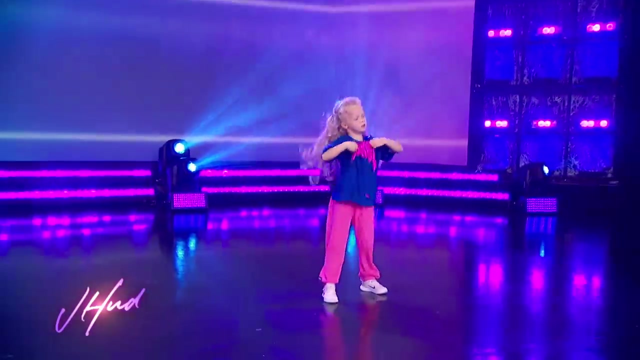 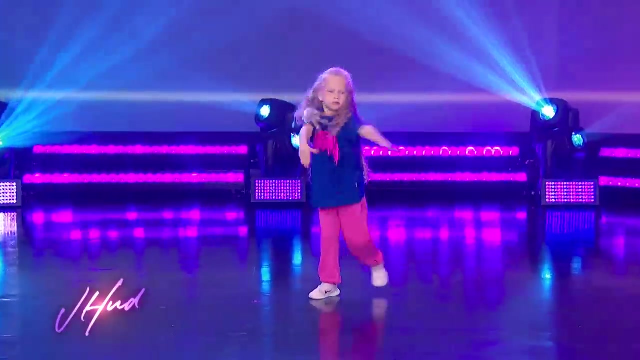